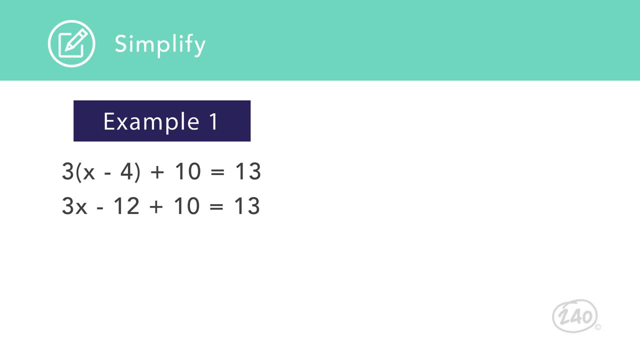 equal sign have an X. However, the values negative 12 and 10 are like terms because they are both constants. That means neither has a variable as part of the term. When negative 12 and 10 are combined, they become negative 2.. In example 2, after the distributive property has been: 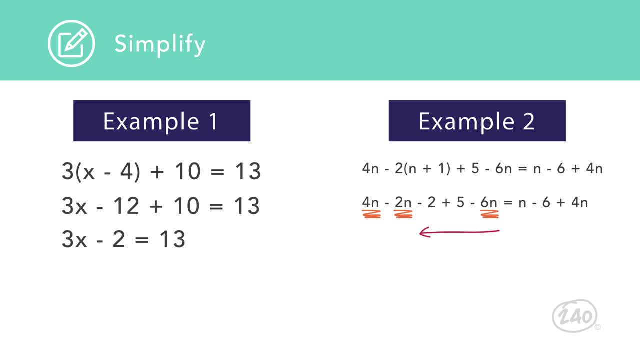 applied. there are three terms with the variable n on the left side of the equal sign and two n terms on the right. It is important to only combine like terms that are on the same side of the equal sign On the left. 4n, negative 2n and negative 6n are combined to give us negative 4n On the 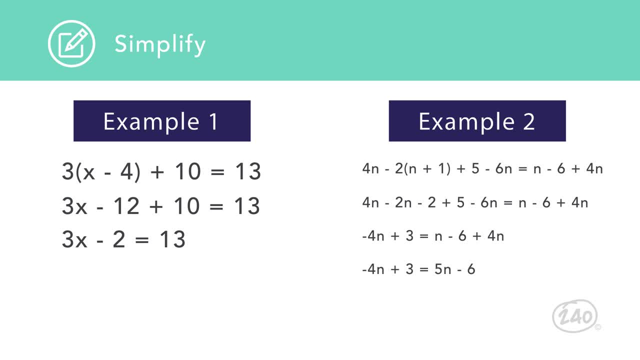 right. combining n and 4n leaves us with 5n. Once each side of an equation has been simplified as much as possible, then the process of solving can begin using inverse operations. Example 1 is solved as a two-step equation: A line drawn down. 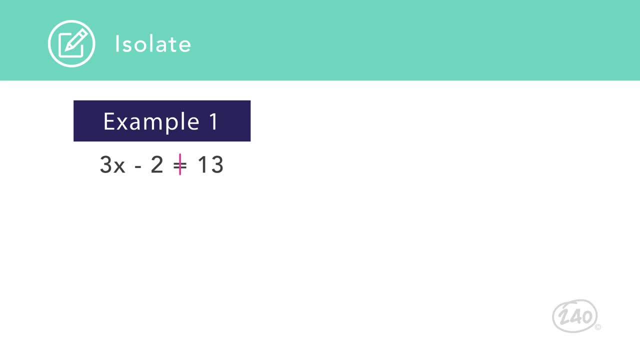 the center of the equal sign reminds us that whatever operation is applied to one side of the equal sign must be applied to the other. In the original equation, X is first multiplied by 3, then 2 is subtracted In order to get us X by. 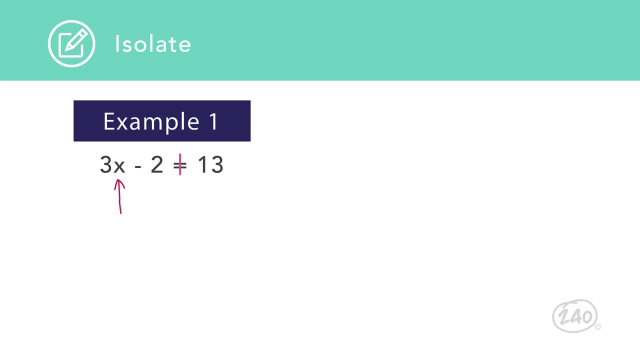 itself apply inverse operations in the reverse order from which they were applied. This means that since the last operation to happen to X was to subtract 2, we must reverse it first by adding 2 to both sides of the equal sign. Next undo. 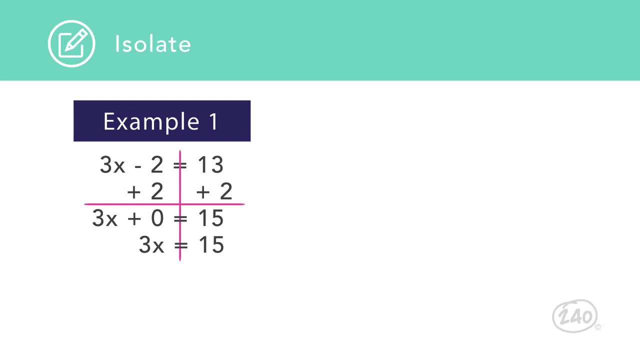 the operation of multiplying X by 3.. The inverse of multiplication is division, so we divide the quantities on both sides of the equal sign by 3.. In other words, when isolating a variable, inverse operations should always be applied in the reverse. 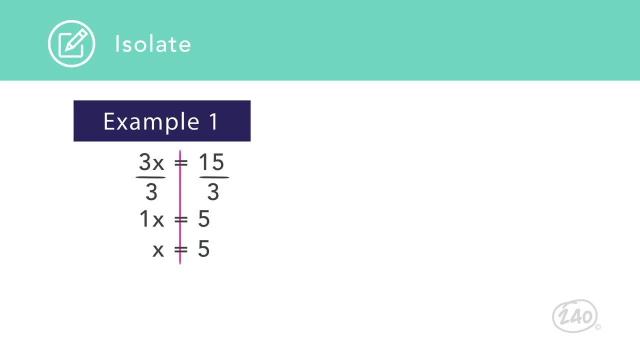 order of operations starting with undoing addition and subtraction and ending with undoing parentheses. Example 2 has variables on both sides of the equal sign. All of the ends must be moved to the same side of the equal sign using inverse operations before you can isolate. 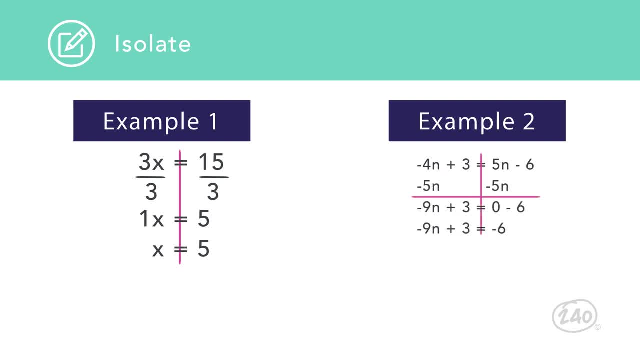 the variable. It doesn't matter which side of the equal sign the variable ends on. Some people prefer to always have the variable on the left of the equal sign and move the variable term from the right to the left. Others prefer to keep the coefficient.